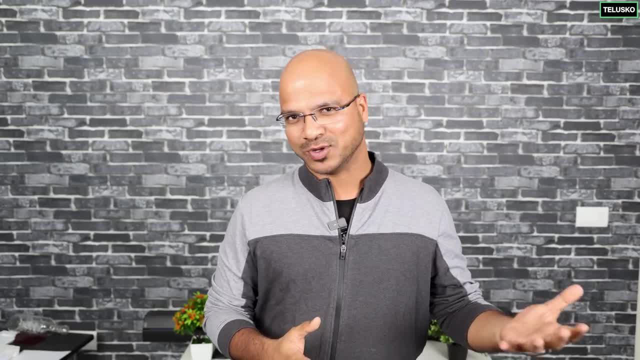 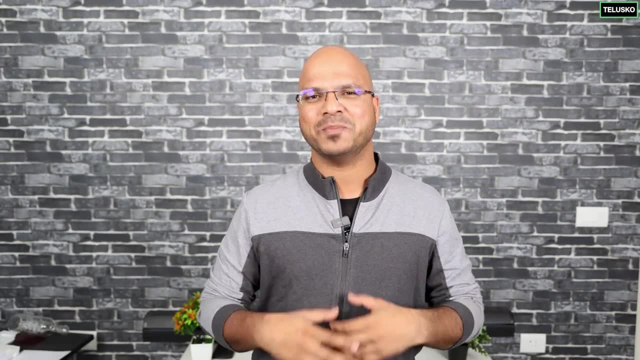 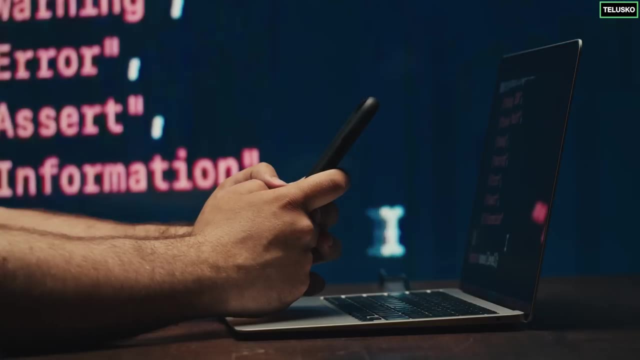 are changing with the AI tools. So the end of last year, basically, we got this new tool called ChatGPT And then, of course, with a great marketing- not by them, but by the people- everyone started talking about ChatGPT. Hey, you know, we don't need developers. now ChatGPT will. 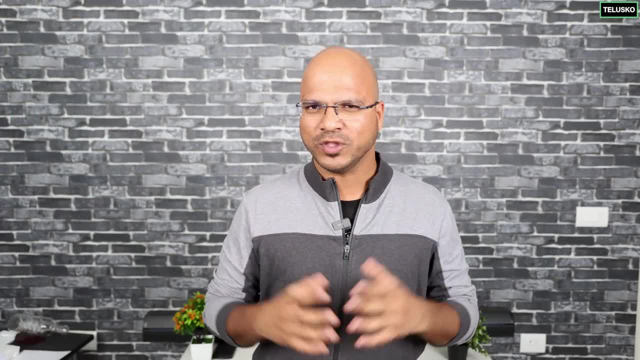 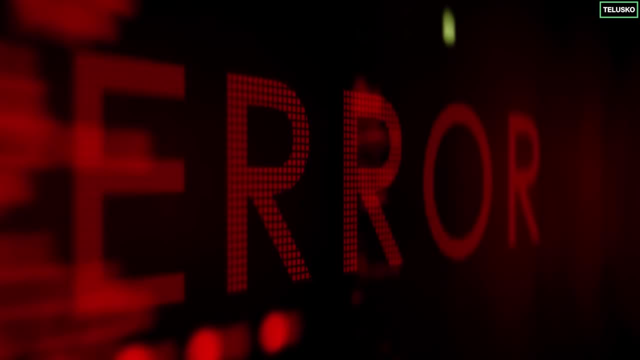 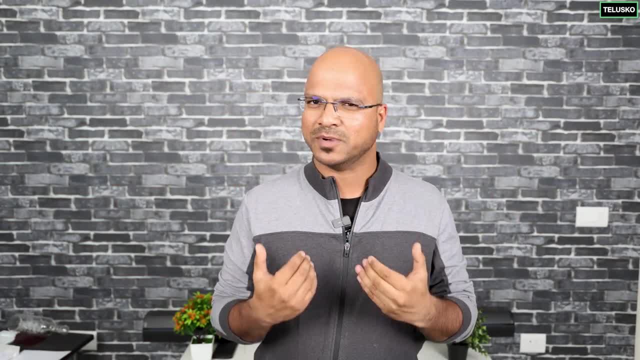 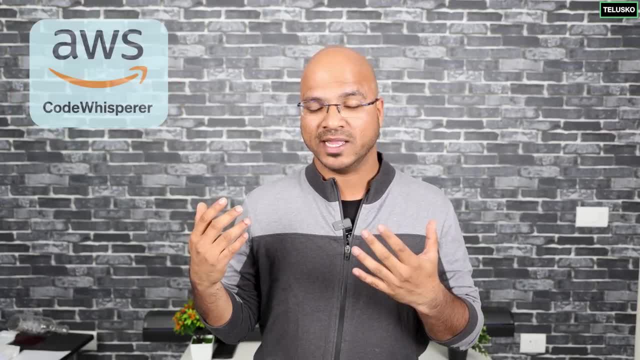 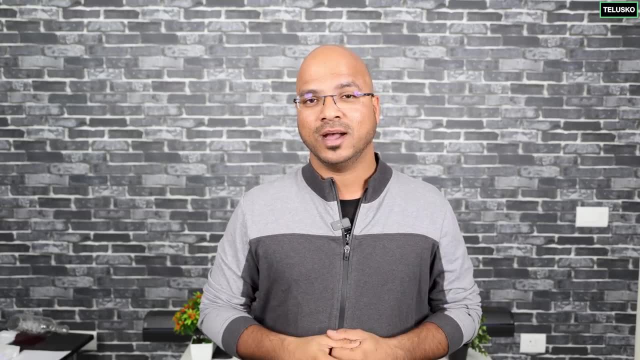 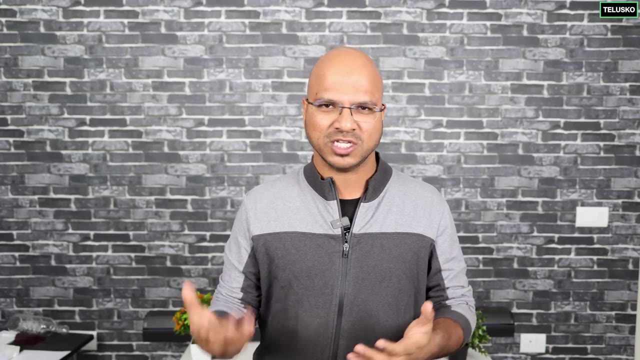 Copilot, Google GitHub Copilot. We got AWS CodeWhisperer. There's so many tools available right which are a part of your IDE Example. I use Copilot a lot with my Intel Azure for development And then it helps me to complete the code. It helps me with the suggestions. And also we got a tool where it will create a uego de mercado. So when you have a project that you want to make, you can do it with intelligence of your own hand. So when you have a project that you want to make, you can do it. 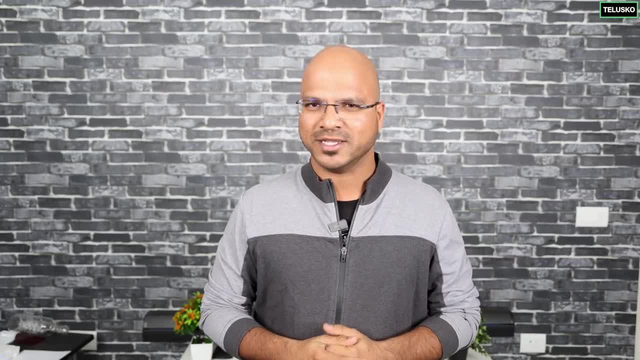 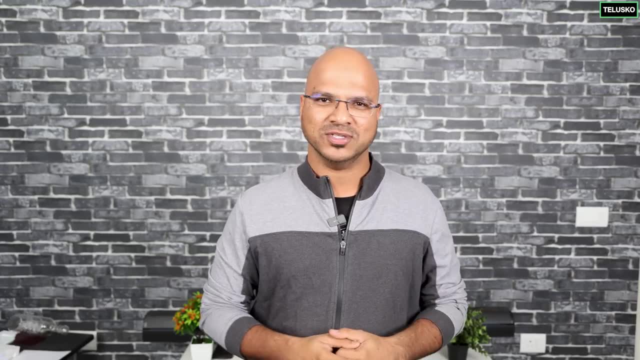 You just give a prompt and it will give you the project. I tried it, but it never works. I have never got a project which works on the first go. I have to make some changes. So is it really replacing developers? Not exactly. 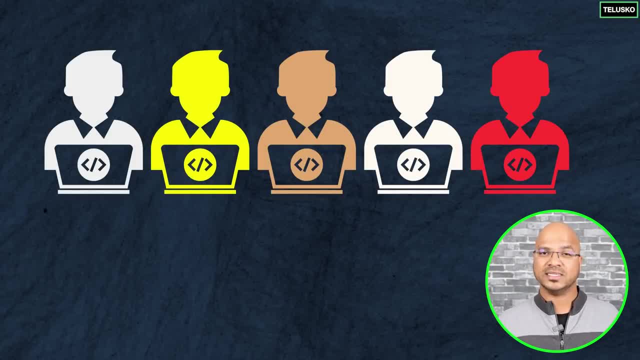 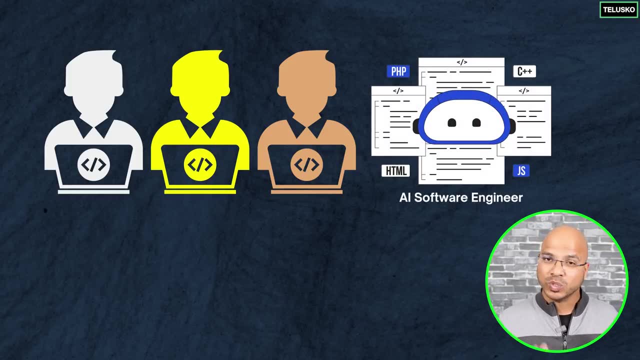 Let's say, if you have a team of five, and now, since AI is helping you, you might need a team of three people, or two in the best case, But the thing is, you need human developers to understand the code given by the AI tools. 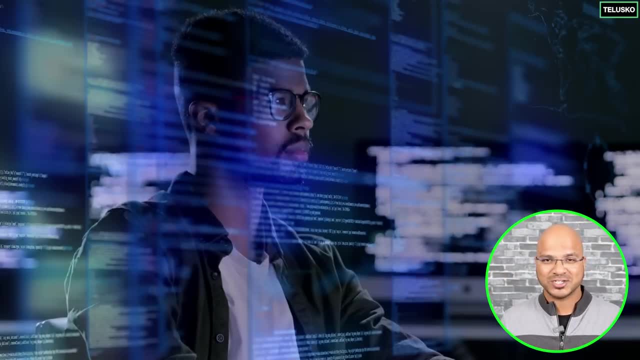 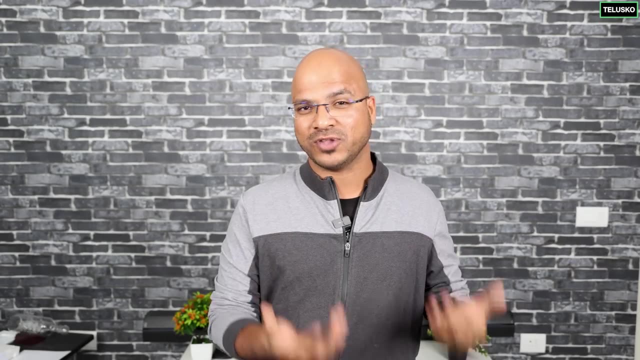 and most of the time they give you weird code which is not structured, which is not even a clean code, and then you have to refactor the entire code to make it work. Ultimately, you're spending enough amount of time. See, as time progresses, it will improve, for sure. 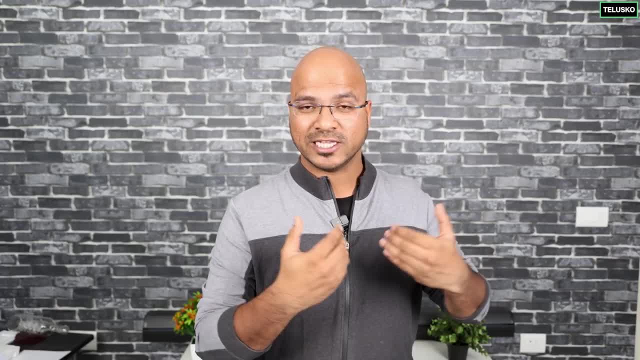 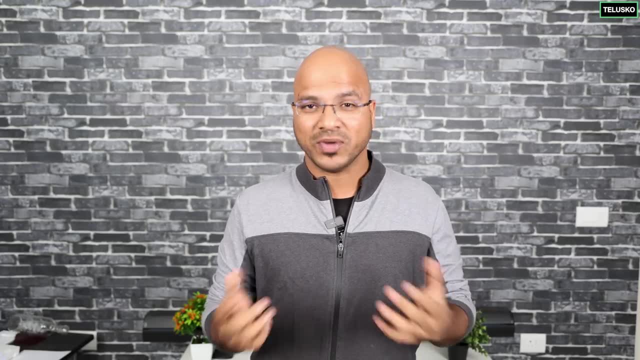 But then with Copilot you can use it and you can make it work. You need an experienced developer who can make the changes. Why I mention experienced developer here is because for a fresher you can write your own code, but then when someone else is giving their code to you, it's difficult. 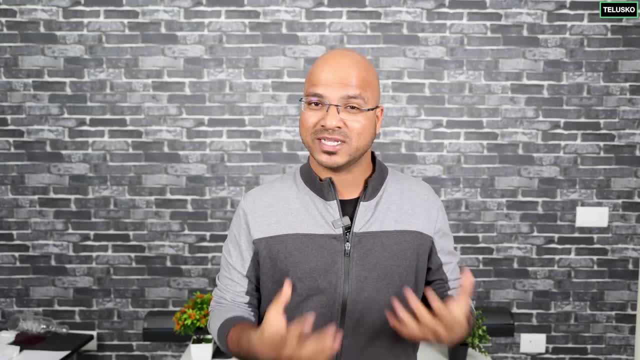 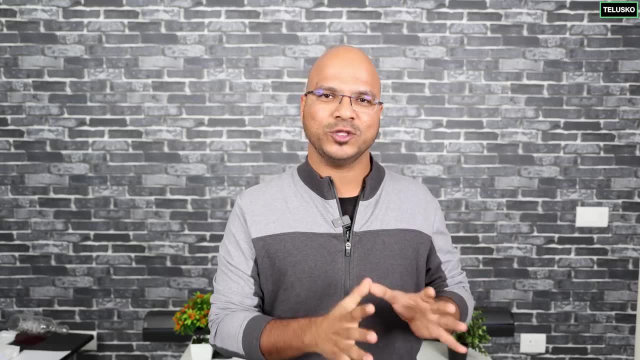 to read for freshers, And that's why it takes some time for freshers to understand others' code. It may take one or two years so you become an experienced developer, But that's the thing, right. Even if you want to use AI tools, you need expertise. 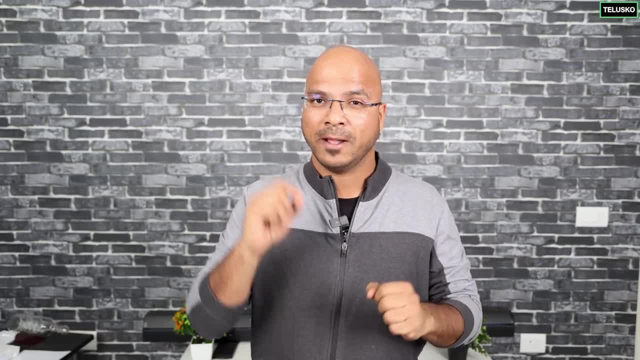 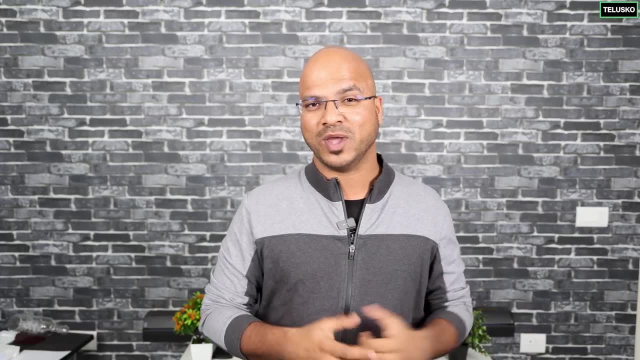 And that's why we were happy with all these AI tools, because they were helping you. But now we got Devin And Devin says okay, so I will give you the code. You'll be saying, hey, we are getting that from other tools as well. 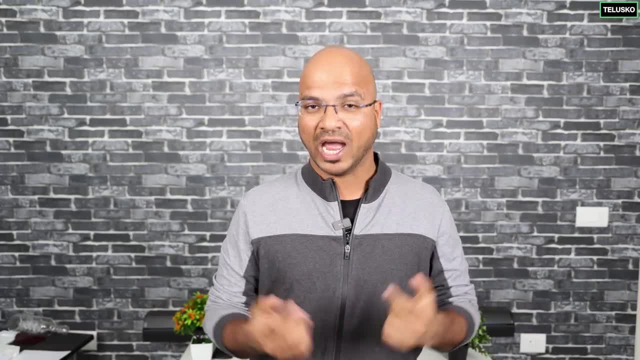 Now Devin says: you don't, You don't even have to debug by yourself, I will do it for you as a human, okay. So example: if you get the error, if you are facing some bugs, what you do. 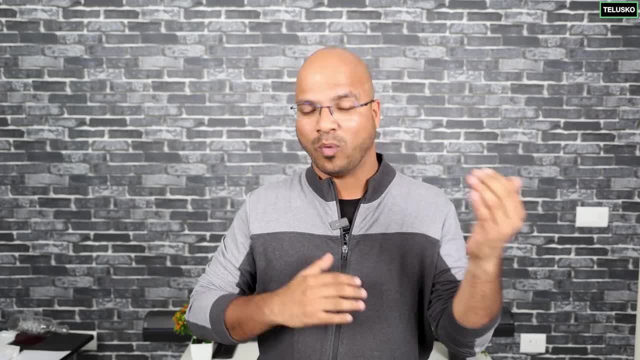 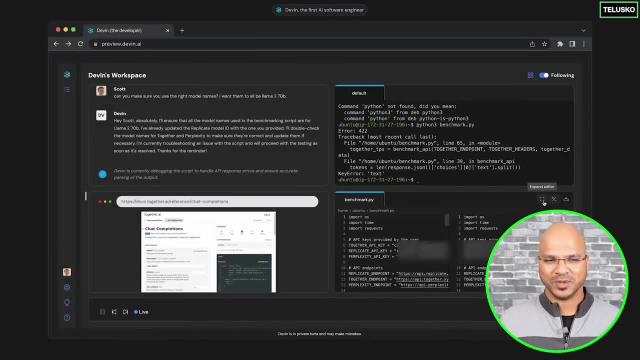 You write println statements to see which function is getting called, what is not getting called, and then you debug it in that way. Devin says: I will do the same thing. And we are a bit concerned now because if Devin can write a code, if Devin can debug, 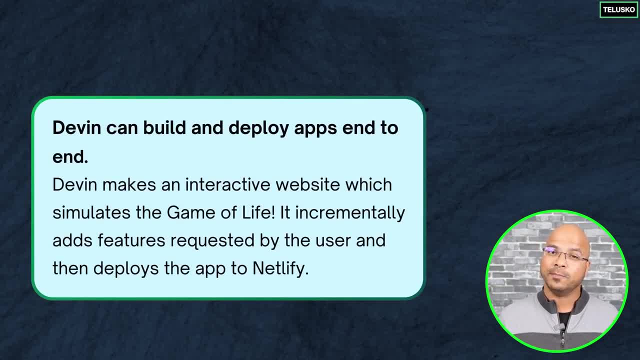 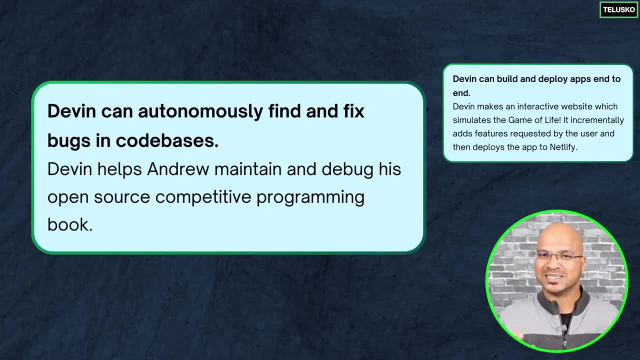 a code. in fact, it also says that they can even deploy the code on the production. They also say that they can find bugs. Find bugs in the open source projects. I mean, this is scary for developers, right, because that's our job. 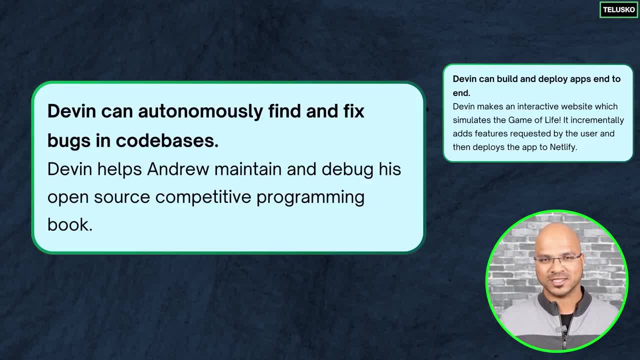 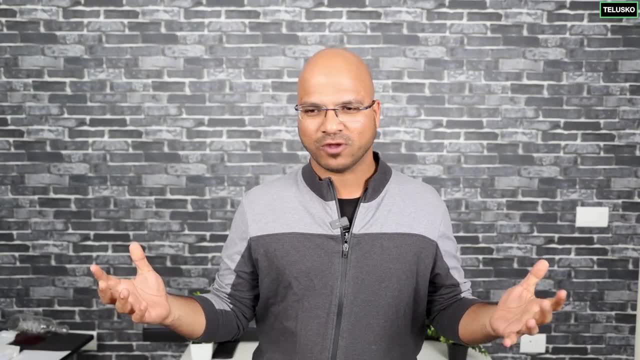 And we are proud of being developers, right, or coders. you can say: But here's the thing: If Devin can do all those things for you, what you will do? Maybe a lot of negative things are happening in the social media by saying they are going. 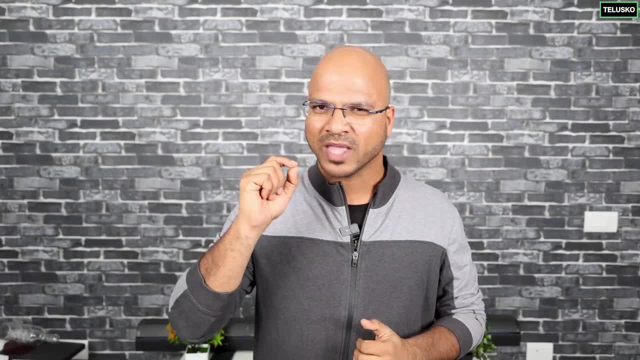 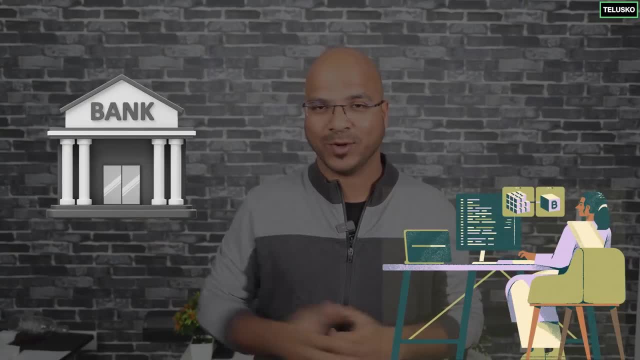 to replace you. you'll be jobless. But here's the thing: Every new technology creates that perception that you are out of job. with blockchain, with cryptocurrencies, All the jobs are going obsolete. With computers: in year 2000,, we thought all the other jobs are going to be obsolete, because 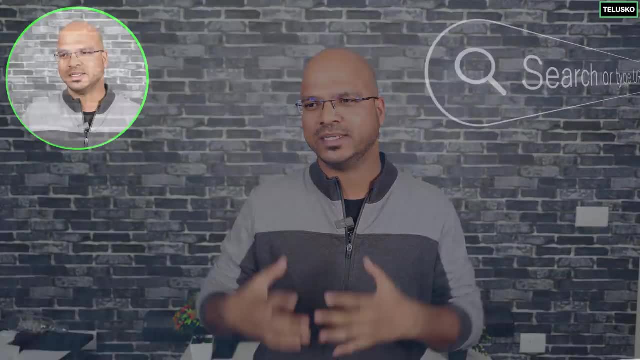 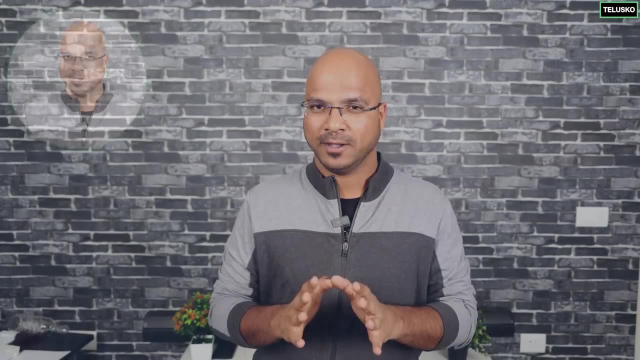 computers can do everything, But no, every time you get a new technology, you get new set of vacancies, you get new set of positions available. right, And with the AI it will be. But still, when you talk about software engineering, it's not about coding. 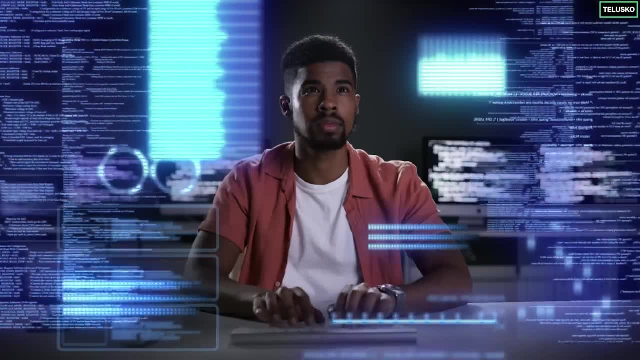 That's one of the biggest misconceptions we have. So if you tell someone you're a software engineer, they directly relate you to code and they are imagining you that the entire day you are working. That's not a good idea. That's not a good idea. 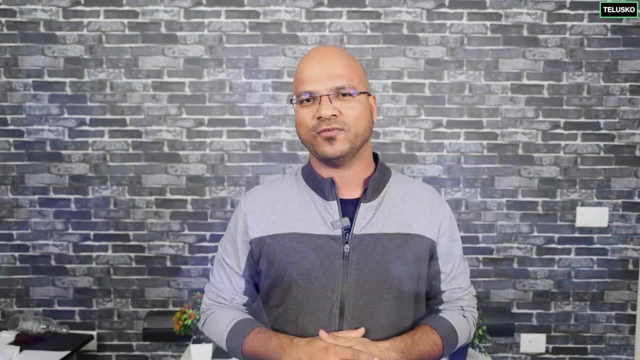 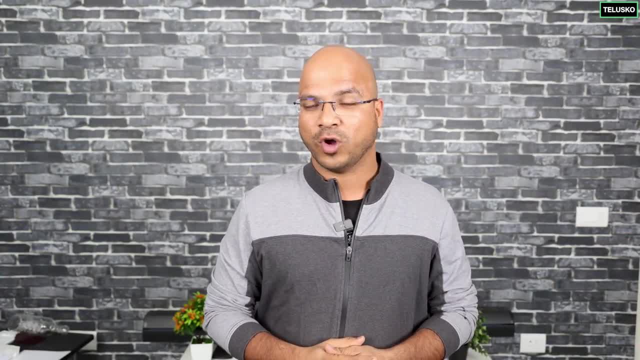 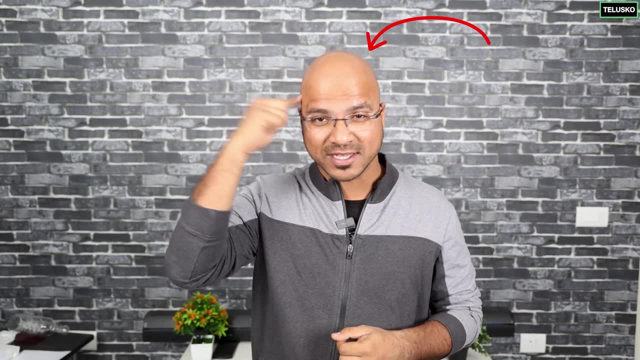 the time. Of course we love writing code, but that's not what we do the entire day. I would say only 20% of our task is actually on keyboard. 80% goes here right, And that's where humans excel. 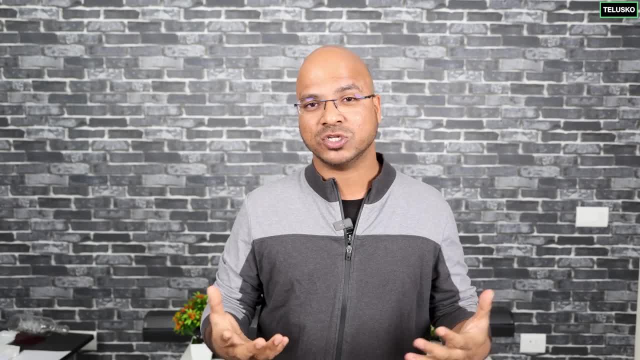 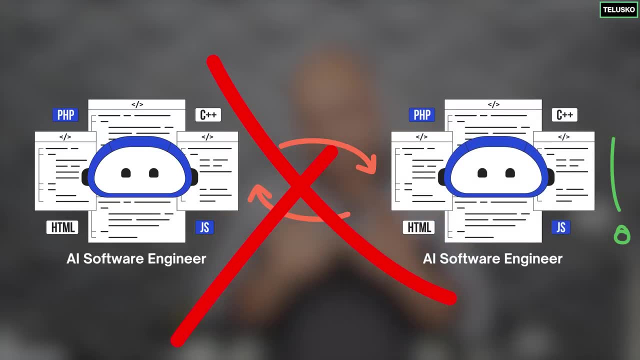 AI can help you with the code, AI can help you debug the application, AI can give you some tips, some suggestions, but it cannot replace the human thinking. yet. I'm saying yet is because I'm not sure. I'm not sure what is going to happen in future, but at this point AI cannot replace in terms 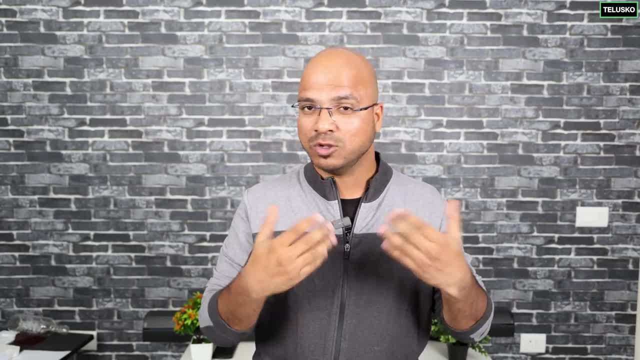 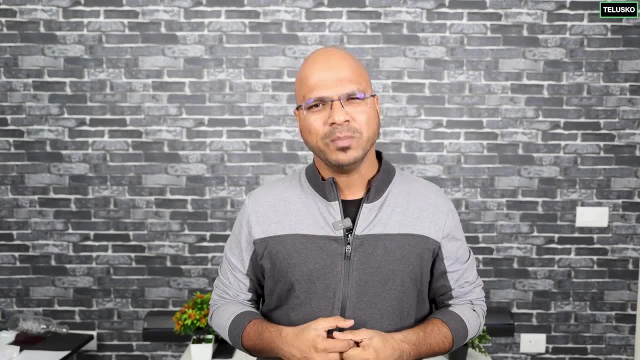 of strategic thinking. See, ultimately, when you build a software or a solution, you give it to your client and your clients are human and only human can think what others human want, And most of the time your client has no idea what they want. 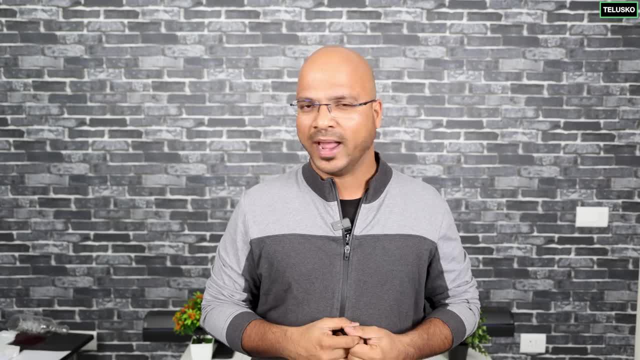 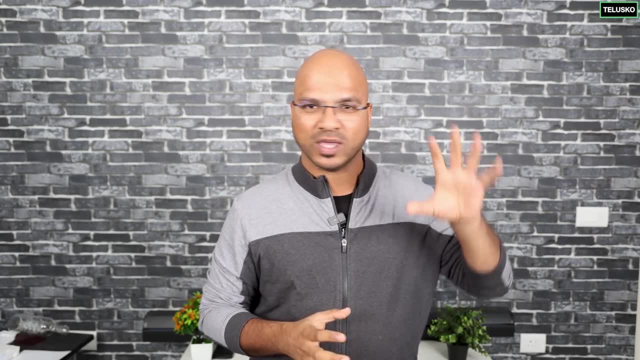 They have a problem, You have to provide a solution to them And most of the time they don't even know the problem. They know there's something wrong, So they will consult with you and they will say: okay, this is a problem. 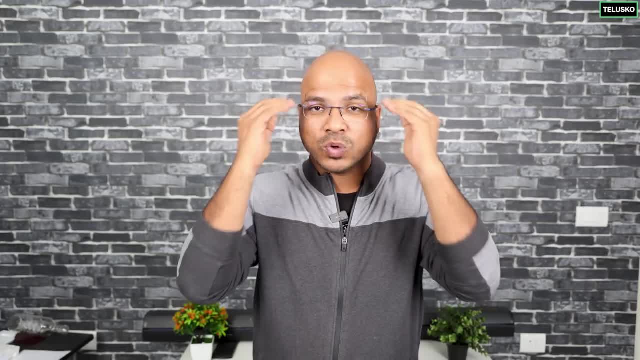 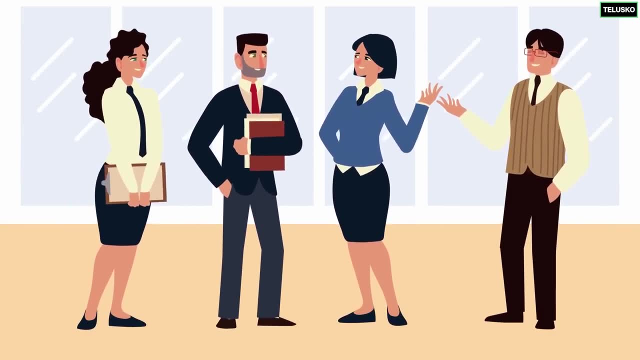 This is something which you are facing. You have to understand the problem. You have to find a solution, on paper, Of course, with your team members, you will discuss and find a solution, And then comes the coding part, which is almost the last part. 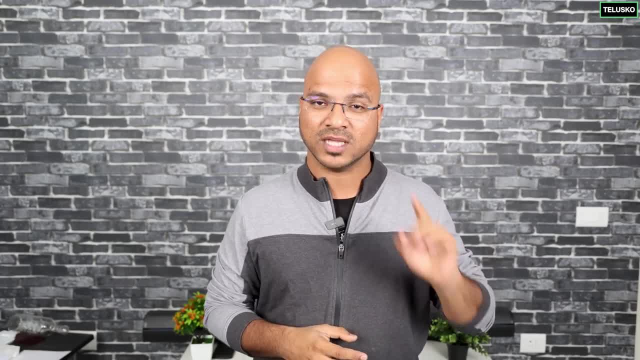 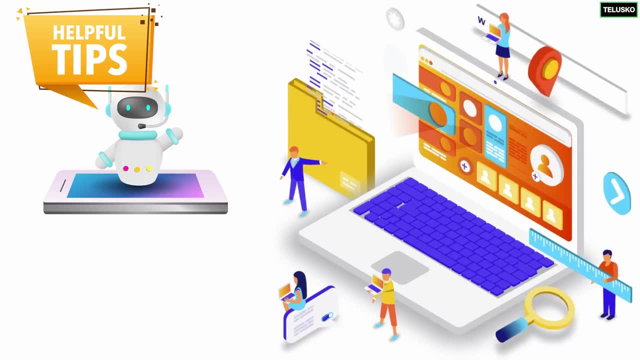 And that's the thing AI can help you with. All the other things are still humans. who will do it? What about the software architecture? AI can give you tips, AI can help you with suggestions, but not the actual architect. There's something called emotions. 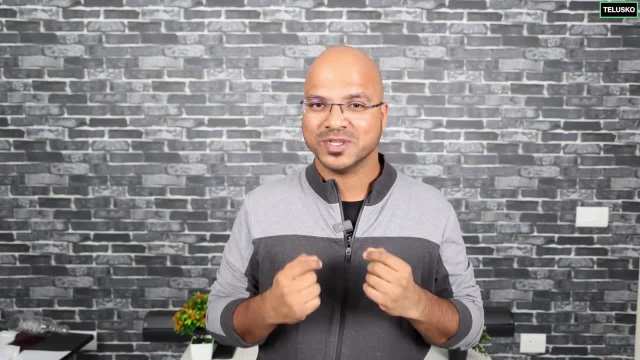 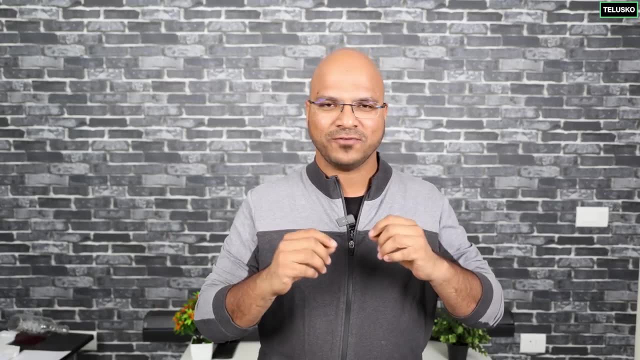 There's something called human, There's something called gut feeling. We humans have that. AI is not programmed to have those feelings. And that's what the problem starts, Because if you see the entire world now, whatever solution you are using, whatever services you are using, 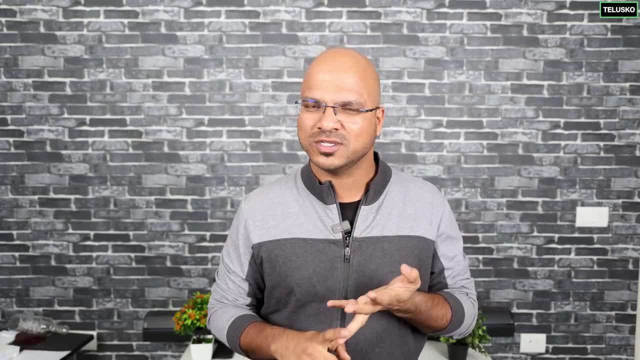 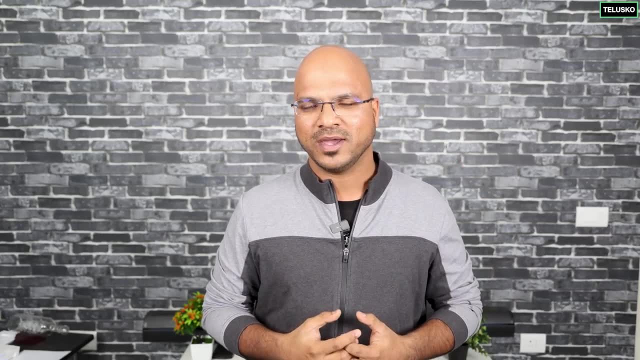 it started, maybe with the help of gut feeling, maybe it's because of some emotions, maybe because of some problem which no one observed. Someone observed the problem and tried to solve it right, And that's the software engineering I'm talking about. 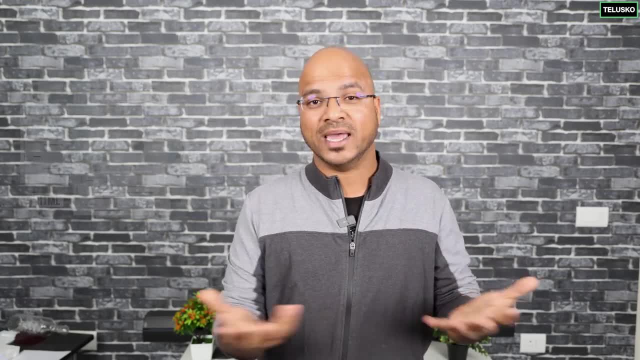 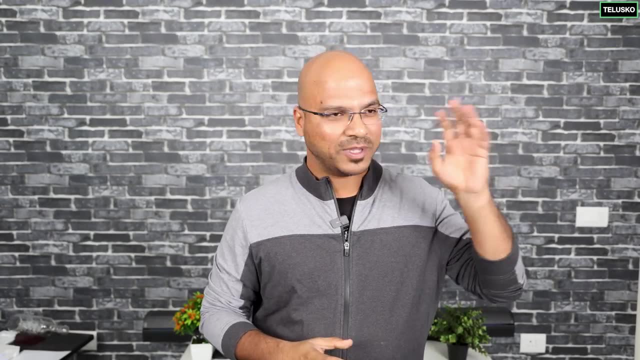 Not the actual coding. So who will code in future? Of course, AI will help you there. Maybe AI will give you the entire software, but you have to understand the problem. You have to understand the architecture, What happens behind the scenes, how the back end is going to be designed. 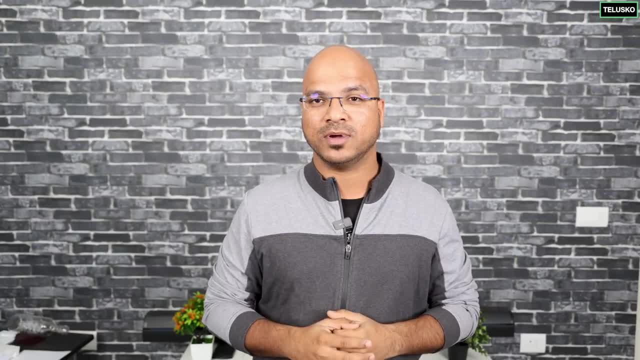 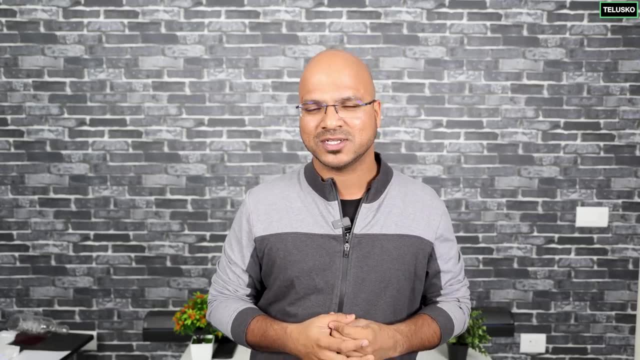 how you are going to scale your application, everything you as a programmer has to define. Now question arise if you're a fresher. of course, most of the problem is with the freshers, because people who are experienced, they have seen a lot of technologies coming up and going. 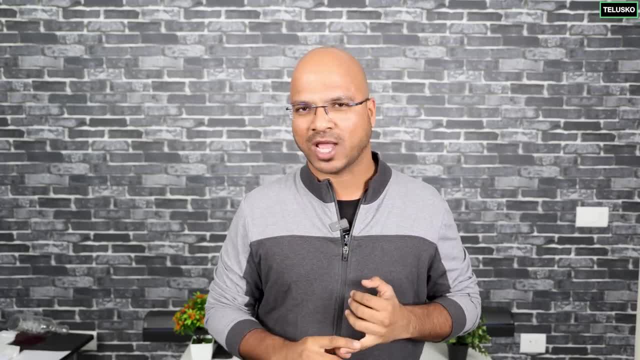 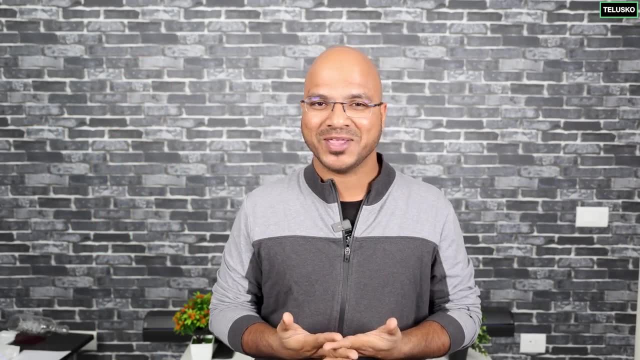 and they have evolved themselves. So, first of all, you as a programmer- it doesn't matter, you are a fresher or experienced- start using AI tools. It's not a competition where you are saying I'm not going to use AI. 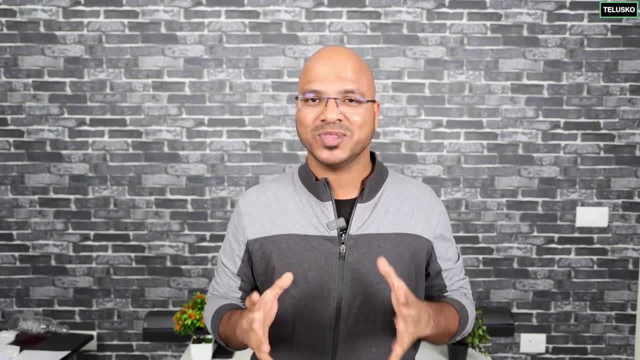 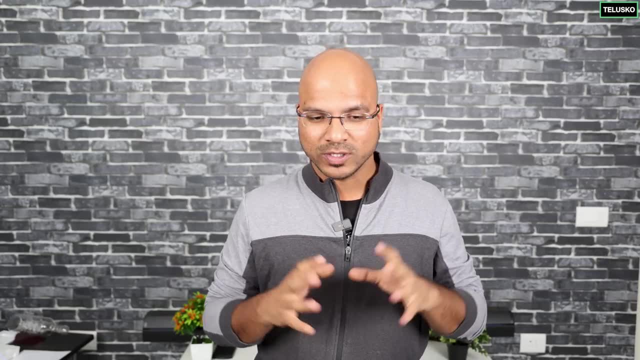 Let me compete with AI. You can't do that. You can't do that. You don't have to compete with AI. You have to use AI. Use it as a tool. Next, don't just stick to a programming language or a framework. 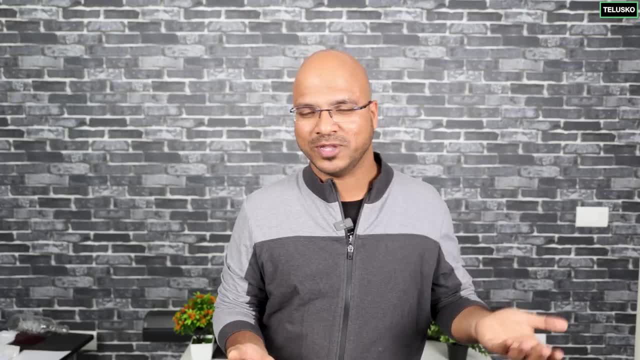 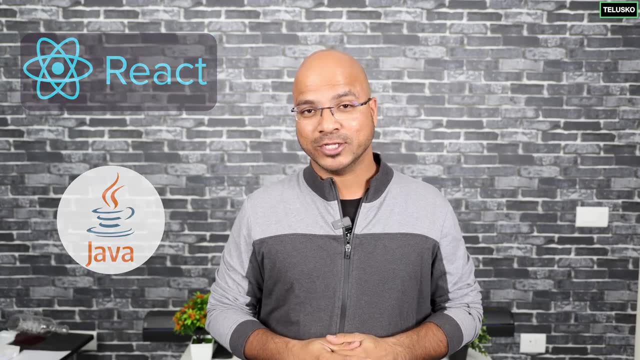 Of course, nowadays, we learn a programming language, we learn a framework. we will update our LinkedIn profile By saying: I'm an expert in React, I'm an expert in Java. Now, that's something. now AI can do What you do extra. 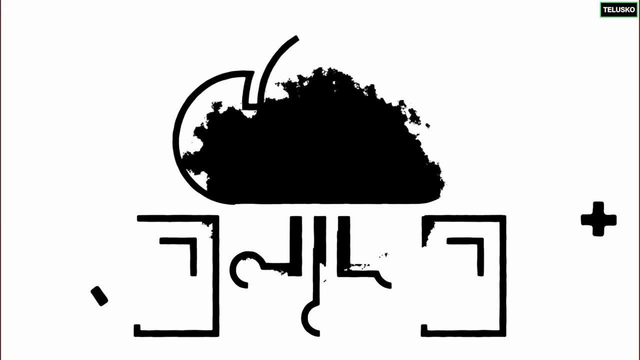 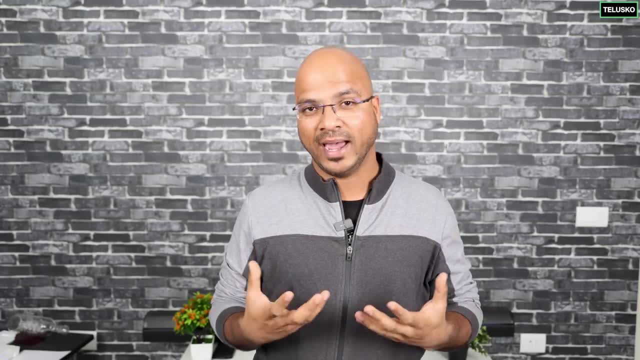 Now that's where you have to upgrade your skill set. Maybe thinking about cloud solutions, thinking about designing an application, thinking about understanding the problem. Those are the things you have to excel at. That means we don't have to learn programming now. 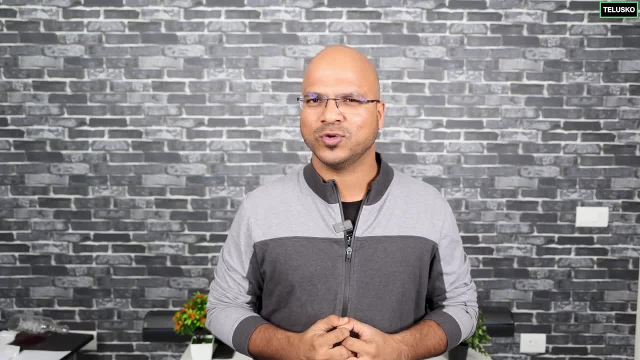 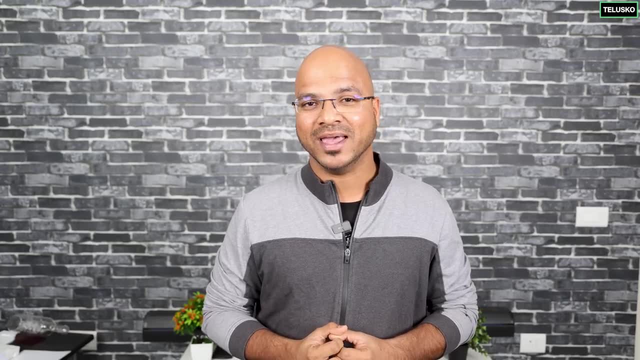 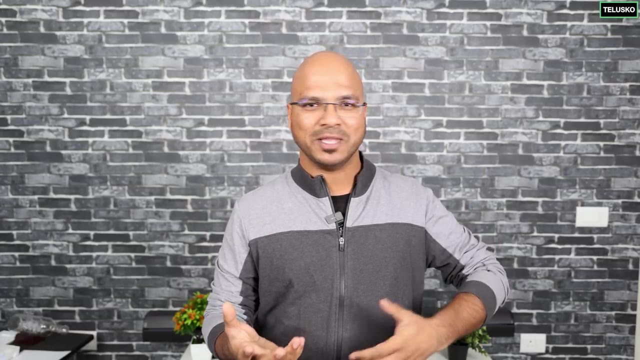 Unfortunately, we still- unfortunately, we still- have to do programming. Reason being: AI will give you solution. You have to learn programming, You have to understand what AI is giving you, And that's very crucial If you can't simply depend upon AI to build a solution and deploy on cloud. 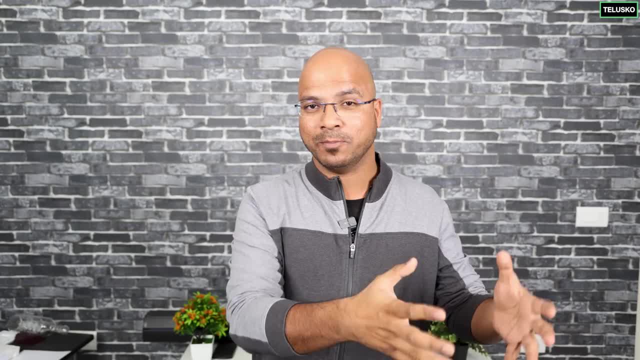 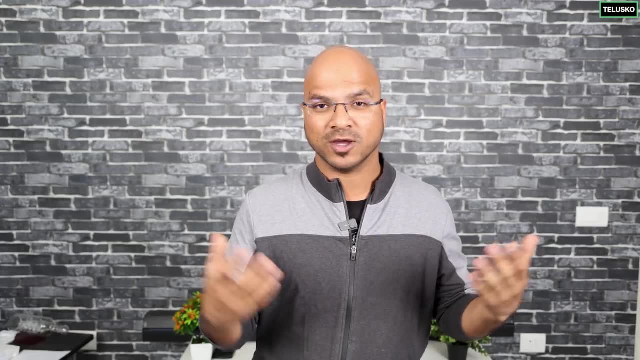 no one will trust it. In fact, most of the companies. they're not even allowing their employees to use ChatGPT or Copilot. It's because their data, they want it to be secure. They don't want to make it public, because AI tools use the data from the client as well. Of course, they are building their own AI tools to make it work. I'm not sure how that will go, because they don't have enough data to train, but still they're not allowing it, And a company will not simply trust AI software and directly interacting with their customers. 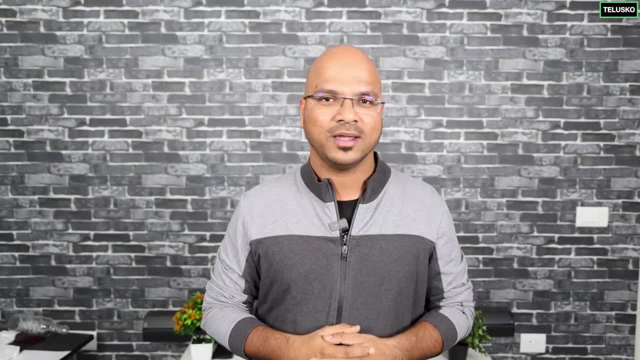 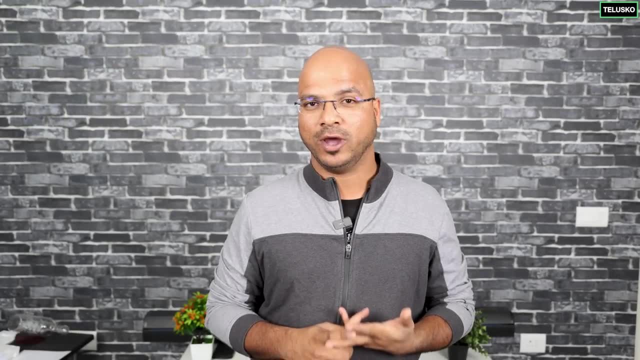 I mean, think about the banks, think about hospitals, all the critical applications. We need humans there, even for deployment, even for building. You can't simply get a solution from AI and you will deploy it, You will check, you will debug. 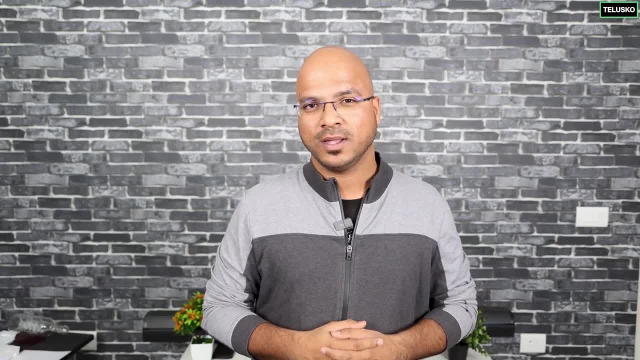 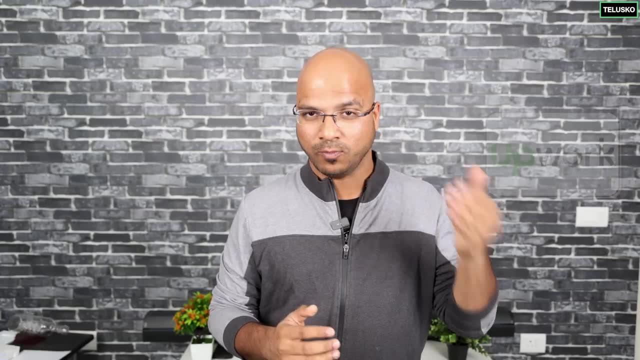 you will refactor it and all the things will be involved there. But what about the startups? What about some freelancing projects? I saw the demo of Devon. It can also create projects which are there on the Upwork of freelancing projects. But see, freelancing projects are not critical applications.